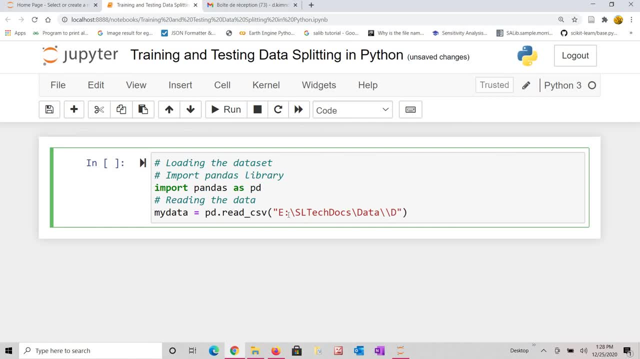 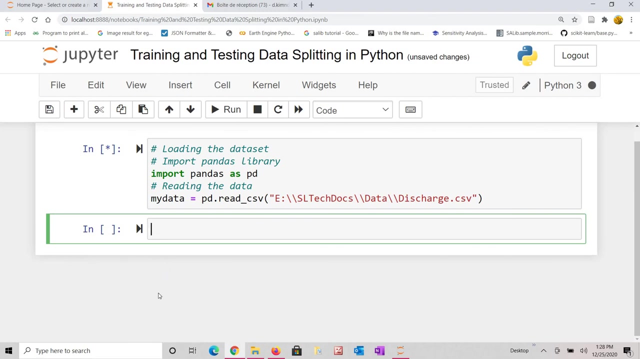 I double the backlashes and I type discharge dot, csv, Double here. Ok, So let us run it. Let us see the data. Let us see the description of the data Data dot describes: Ok, This is the data we have. 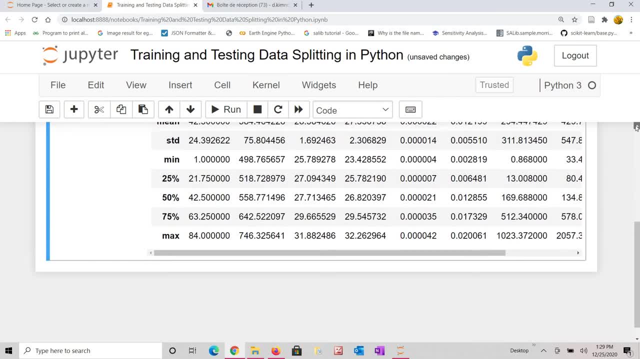 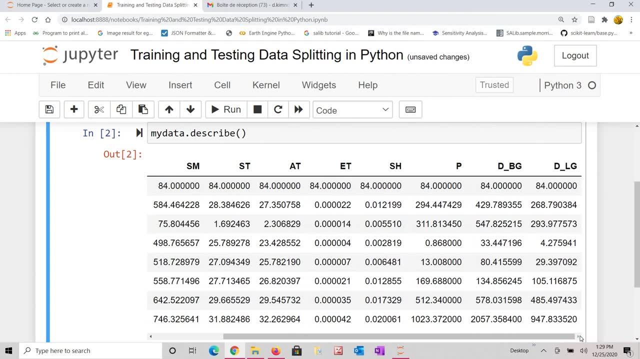 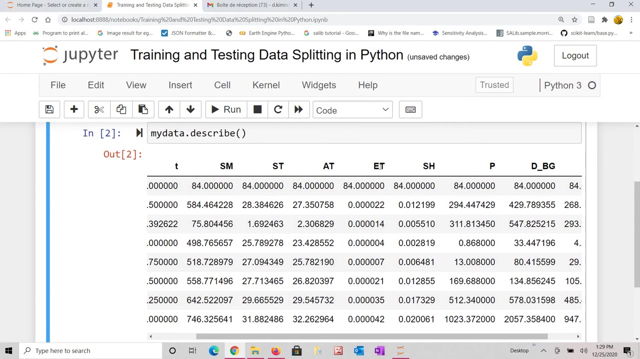 With these columns. So we have D for discharge. So discharge at two locations, BG and at LD, And we have precipitation. We start with soil moisture. The time is here, also Soil moisture, Soil temperature, Air temperature, Evapotranspiration. 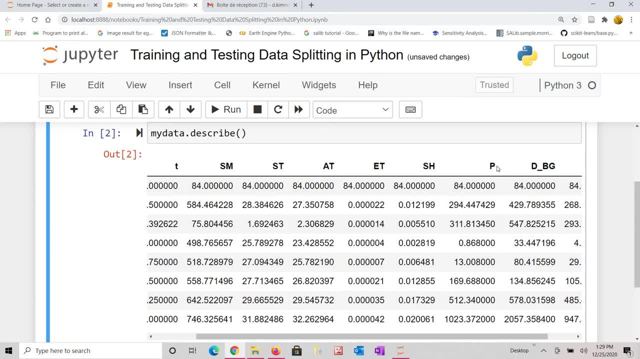 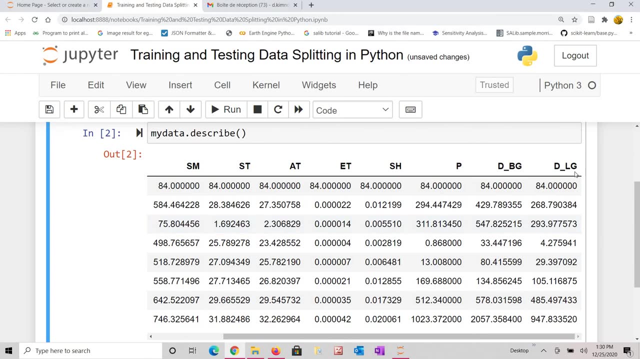 SH, Specific humidity, P precipitation. So these six variables are the input data And the discharge, River discharge. let me be precise: River discharge is the output data. So for modeling purposes, we need to split. I am going to take one. 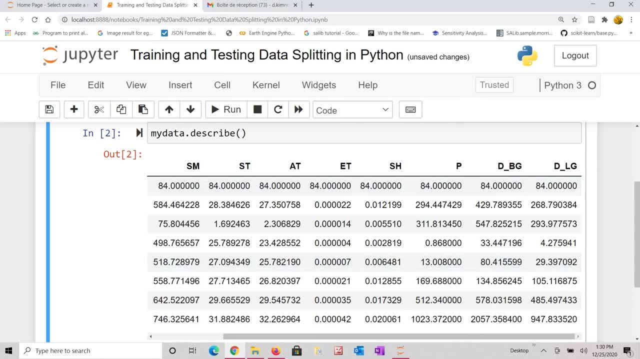 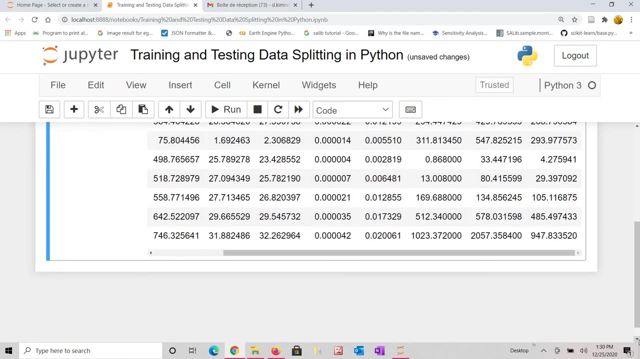 Input data: The soil moisture, SM, And the river discharge at this location- BG- As the output data. So we have X as SM And the discharge BG is our Y. So we are going now to provide the input and output data. 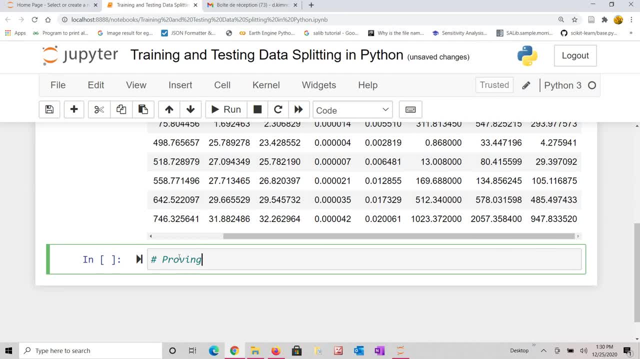 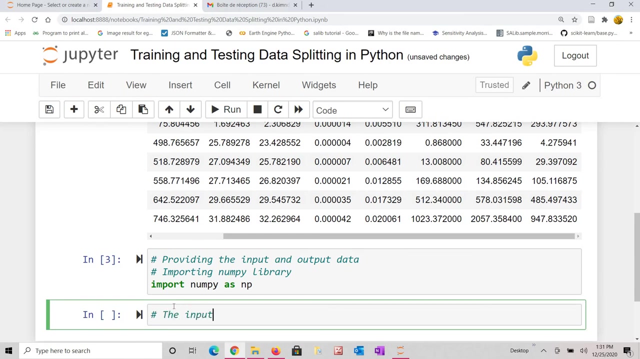 Provide the input and output data, So there must be arrays. So for this purpose, we need to import the numpy library. So Import Numpy as N X. Give us the arrays. Now let's specify our input data. It's X. 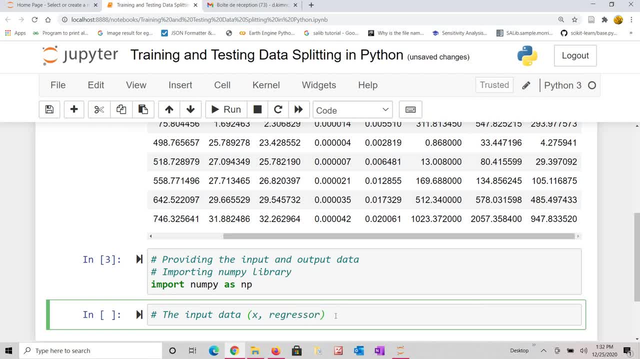 We call it also regressor. So Let me Okay. X equal N, P Dot Array, Parentheses my data. We are going to take SM Soil moisture. Oh Sorry, I should rather take the bracket. 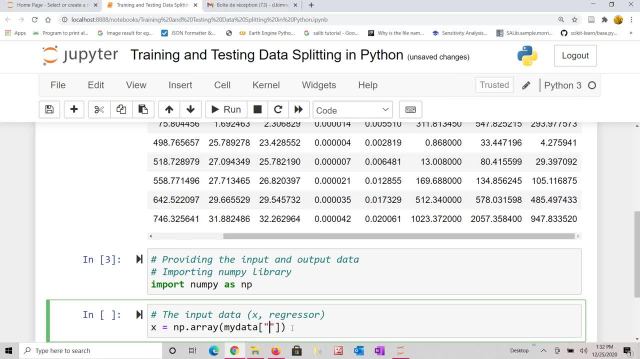 Instead of curry bracket. Okay, SM same. then we need X to be a two-dimensional array, means a colon and several rows, so for this we need to use this function. the shape and the argument minus one to one- so this is minus one to one- is going to give us the two D array. 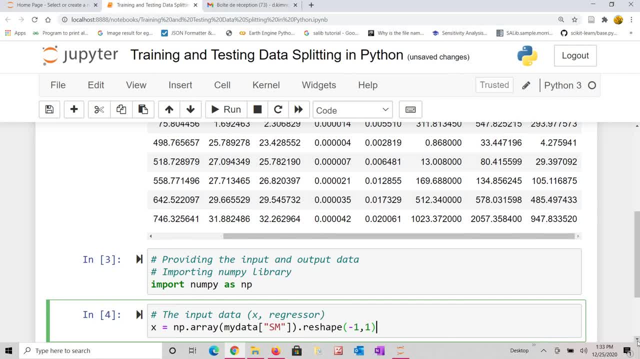 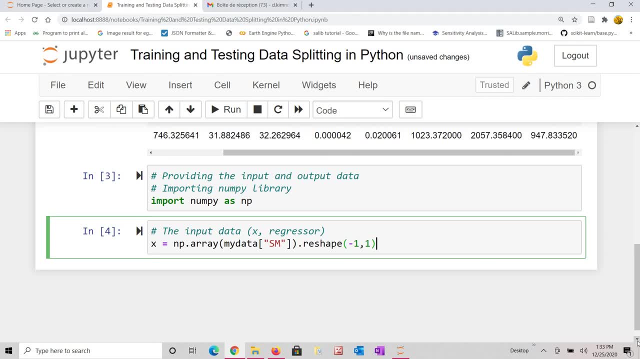 so it is a mass. it must be a two-dimensional array. so we run it and then let's see the shape of our X. it's not shape, or the lower X. so we have a h1 rows and one column. ok, so let's write input, now the output data. let's specify the output data. 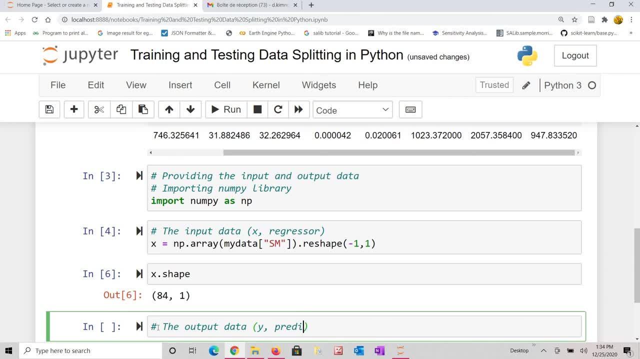 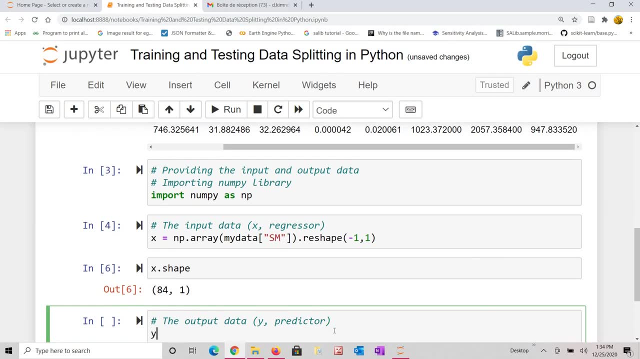 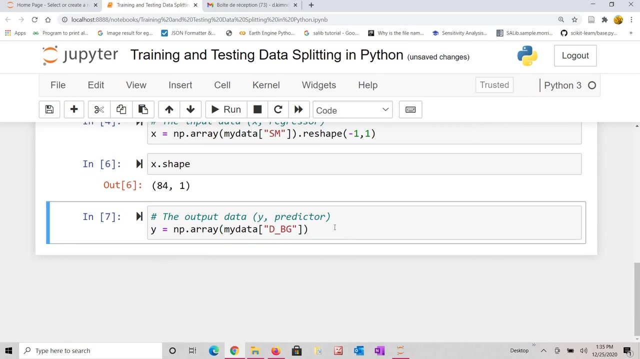 we call it while, and it is a predictor- y equal must be a number, also my data, the brackets in it. as I said, I'm going to take the river discharge at the location called BG And the y can be a two-dimensional array or not. let's find the reply. 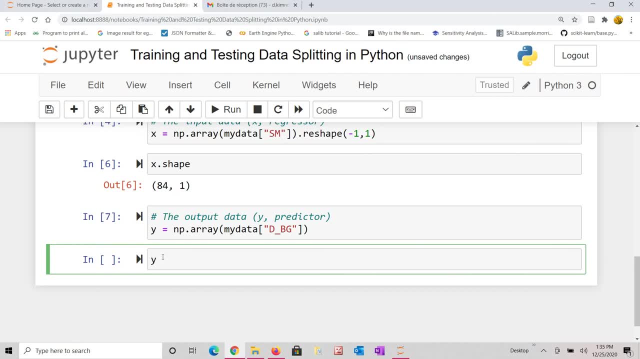 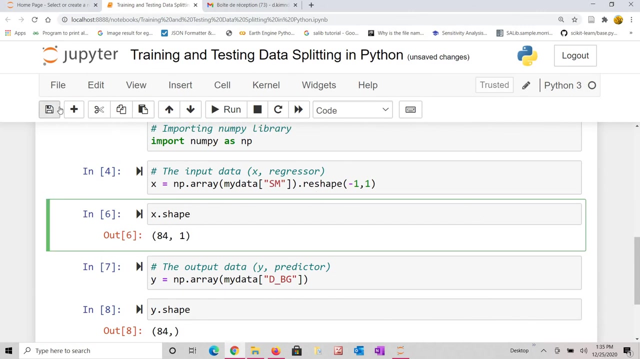 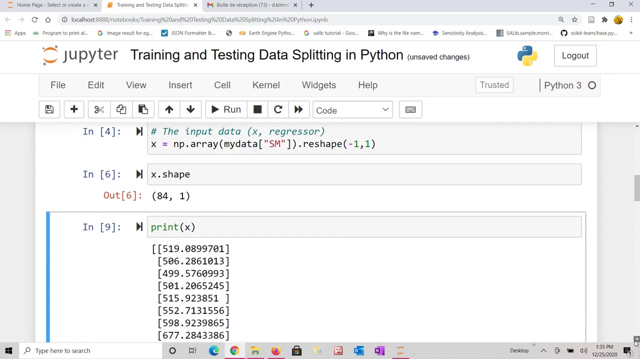 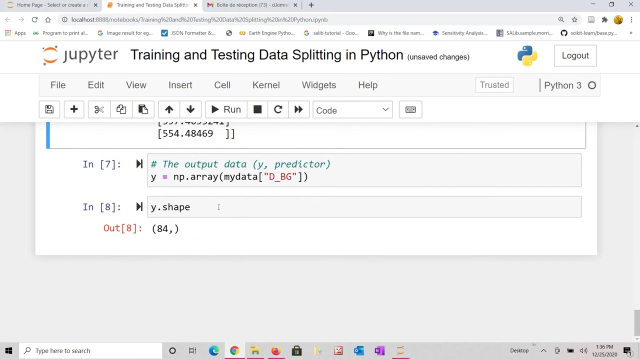 Let's see the shape of y. Write that shape. h1, rose. Let's print them. you see, let's insert a row here to print x. this is x you have. Okay, We print also y and c. 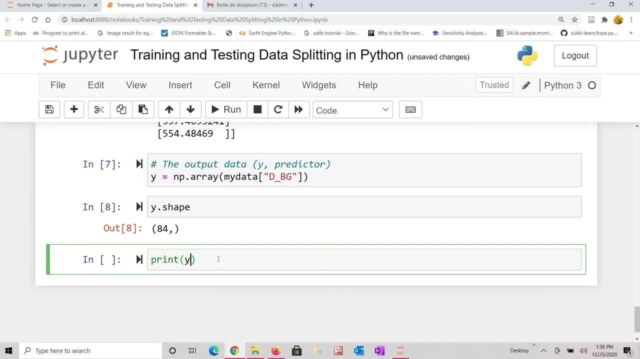 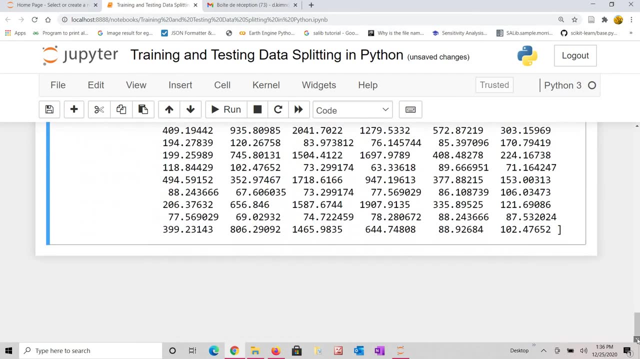 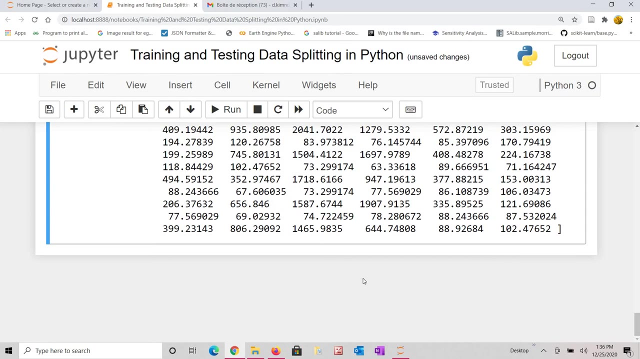 Okay, Okay, Now we are going. let's see also the type of y and the type of x. Type Of x: NumPy class, numpyindarray. Let's change it into y. Type of y: The same thing. 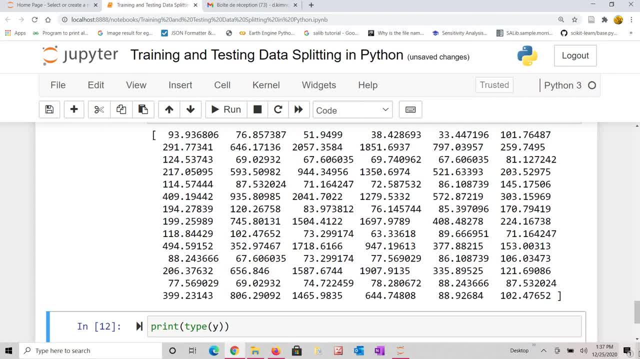 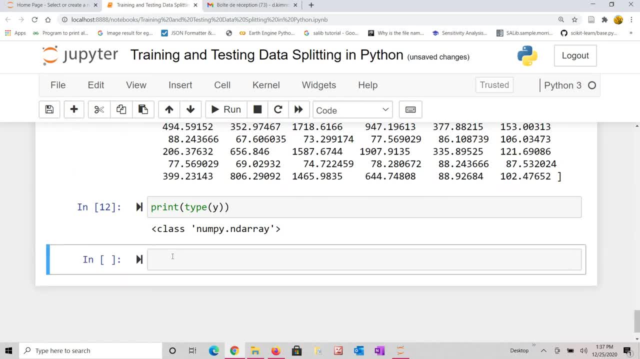 Okay, Now that we have specified our input and output data, the regressor and the predictor x and y, we are going to split The data Data set into train and test. The first thing we need to do is to import the function train test split. 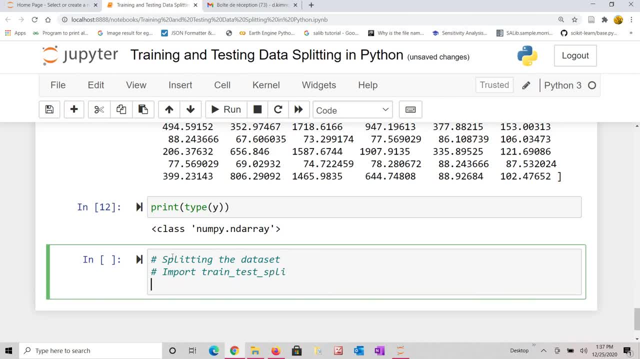 Then we need to import the function train test. You can download it from our browser. So we are going to import the function train test From sklearn, So from sklearnmode selection. Another underscore selection: Import Train Test Ctl. 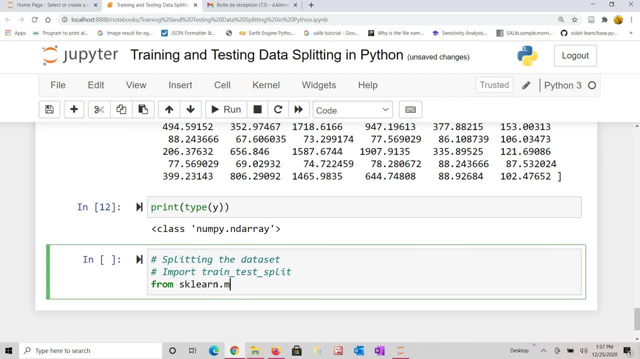 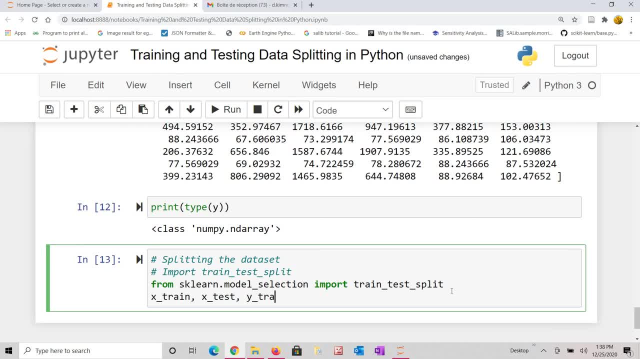 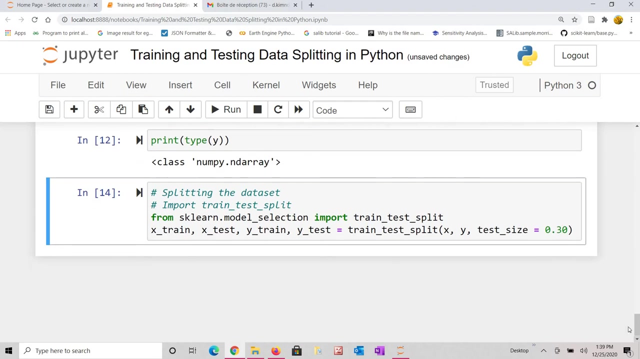 Y train Y test equal. the function train sorry test split X Y test: underscore size equal. let's say we take 30% as test set and 70% as training data set. ok, now we are going to explore the contain we go with. let's start with. 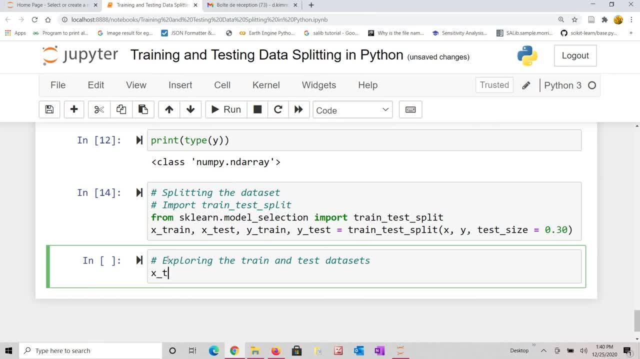 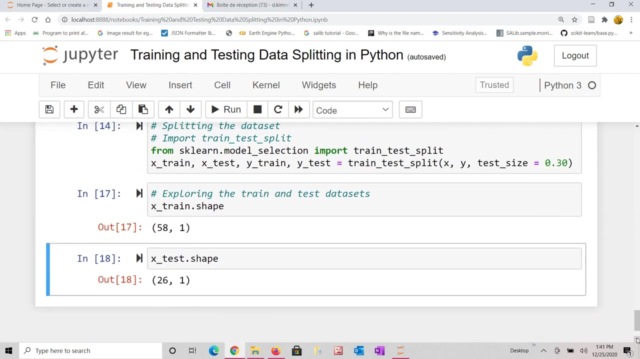 X train- sorry, dot shape. we have 58 out of the 84. let's see X dot shape 84. so the X train is 58 out of the. ok, let's see X test dot shape 26 out of the 84, so 84 minus. 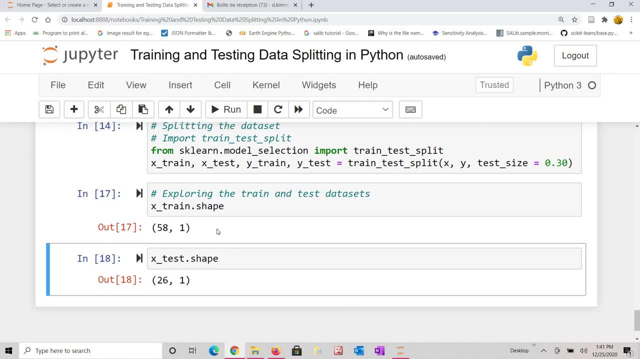 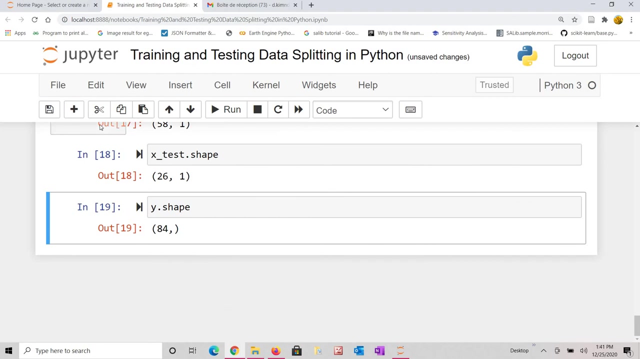 58, 26, so 30%. we do the same for Y, Y dot shape 84, 84. so for Y train, Y test we are going to have 58 and 26 as well. you can use the function print to get the same.